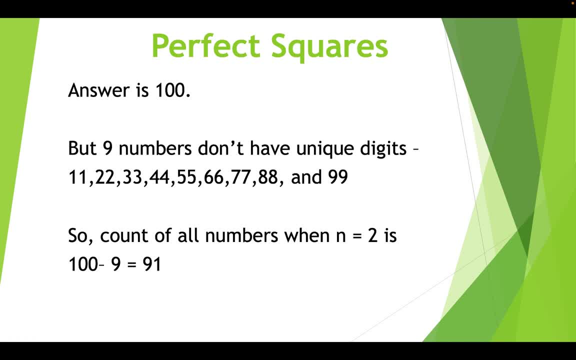 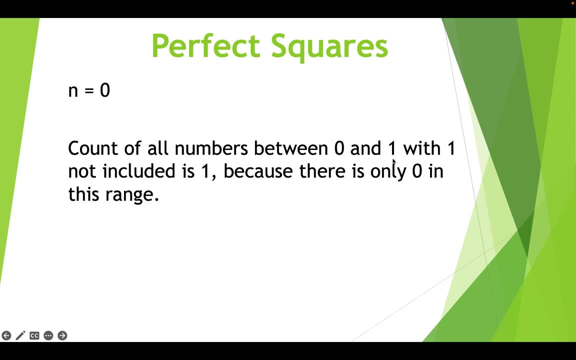 eighty, eight and ninety, nine, because they don't have unique digits. So that's nine subtracted from 100.. So what becomes the count of all numbers when n is equal to two? Ninety one Now. when n is zero, then the count of all numbers between zero and one, with one not included, is going to be one. 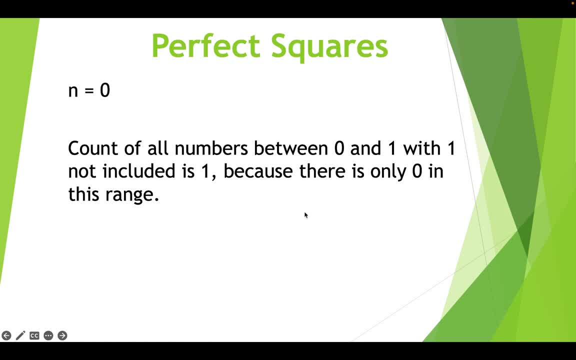 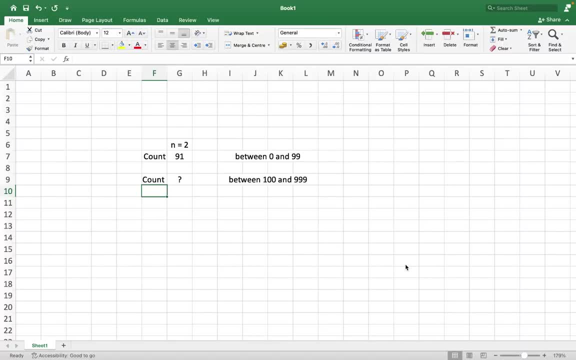 because there exists only zero in this range. right, I am sure you have got the problem statement now, So let's begin understanding the intuition. You have already seen how we found out: the number 91 for n equals to two. So now we need to think on. 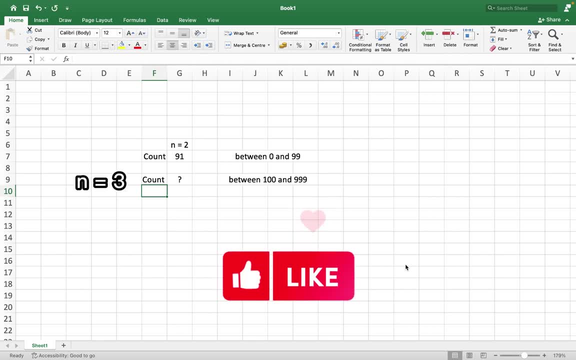 n equals to three. We already know that between zero and 99, there are 91 numbers with unique digits. We need to find out the count of numbers with unique digits between 100 and 999,. right, Whatever the count comes out of all numbers with unique digits between 100 and 999, we'll add 91. 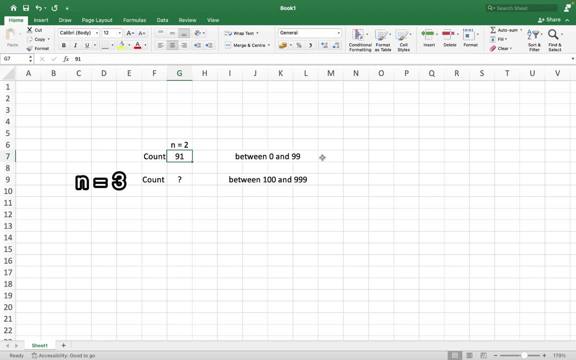 to it and that will give us the answer. The first thing that is intuitive is the count of numbers between 100 and 999 will be in three digits. That's super obvious, right? Since it's a three digit number, it will have a hundred. 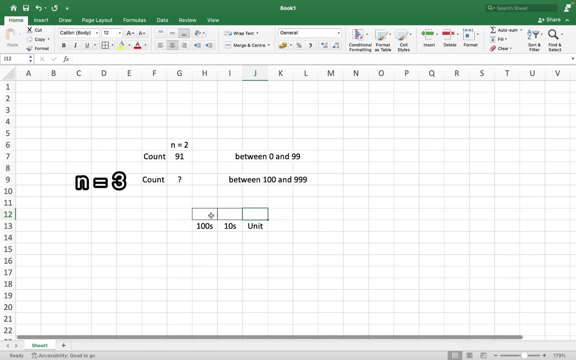 digit, a ten digit and a unit digit. So how many possibilities exist for the hundred digit? Any number between one and nine? Yes, we can't have zero right? So nine possibilities exist. All right, Let's move to three. 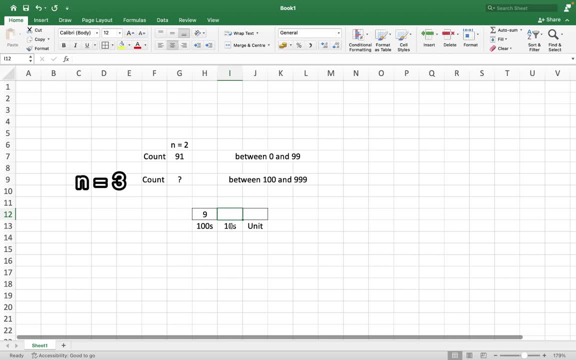 For the tens digit. how many possibilities do we have for this digit? I took a hunch on nine, but then I realized that it can't be, because we are dealing with unique digits, So one digit which is at hundreds place should not be considered. So I reduced nine by one. 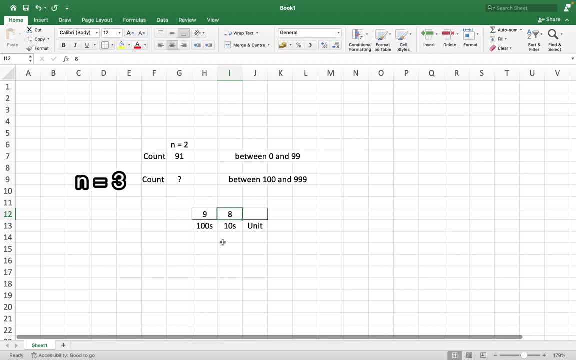 and put eight over here, But wait a minute for the tens digit. we can also include zero, right, You can't have zero. You can have zero at the hundreds place, but you can have zero over here. So the number of possibilities again increases to nine. Okay, And that is what the right number of possibilities? 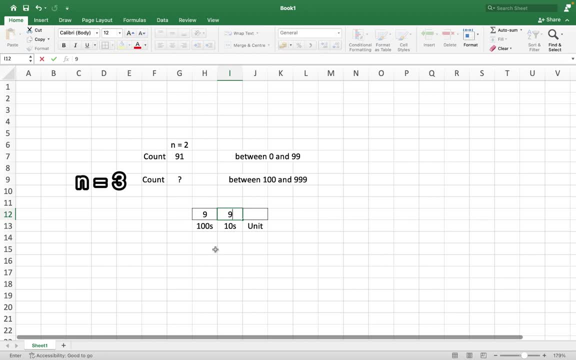 is for the tens digit. All right, We have got two candidates. Let's focus on the third one now. So how many possibilities do we have? We have numbers from zero to nine, which makes it 10 possibilities, But we need to reduce. 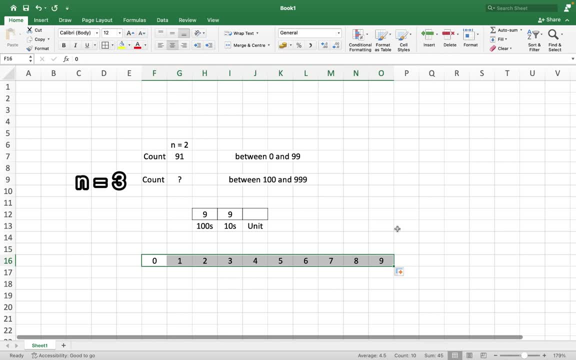 We need to reduce the number 10 by one for this digit over here and one for this digit over here, So that brings us to eight. In simple words, this place can't have a digit that is over here and the digit that is over here. 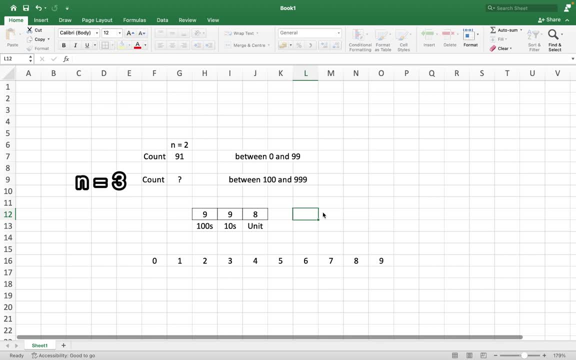 All right, So I put eight over here. So the count is going to be nine multiplied by nine multiplied by eight, That gives us 648.. And we add a 91 to it. From here we get 739.. And that's the count. 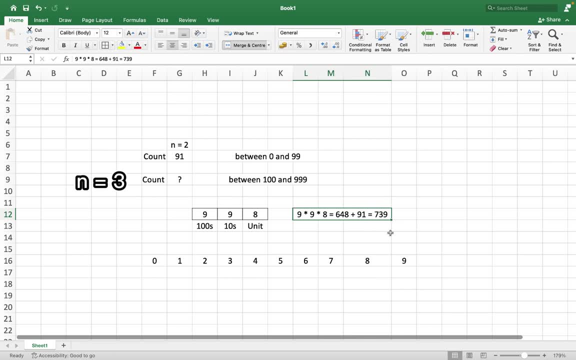 of all numbers with unique digits, for n equals to three. So if we take into account n equals to four, then the count becomes nine multiplied by nine, multiplied by eight, multiplied by seven. Now, if we go back to n equals to two, then let's see if we can find out how many. 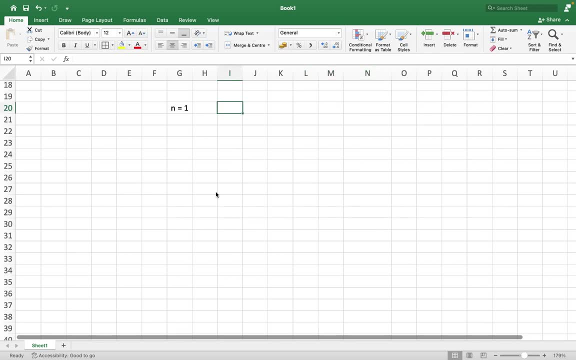 unique digits there are in the number 91, using the same formula. So we know, for, n equals to one. what's the count of unique digits? It's simple: 10, right Numbers from zero to nine. Okay, Now between 10 and 99, if we need to find the count of numbers with unique 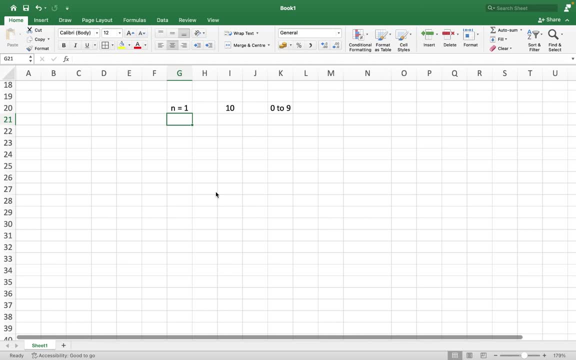 digits, then this is super obvious that it's going to be a two digit number. Okay, So what's the possibility For this 10 digit? nine again, right, Numbers from one to nine, excluding zero. we can't have zero over here. And what's the possibility for this unit digit? Nine again. we just saw. 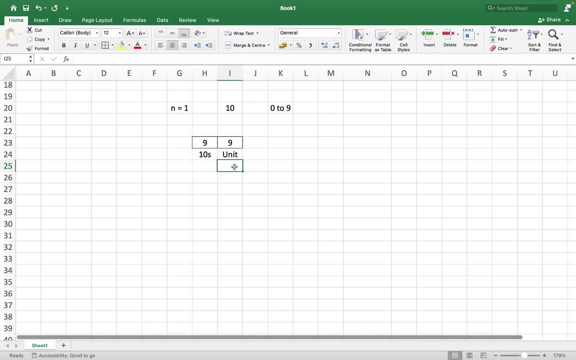 how we populated nine over here, for n equals to three. So this gives us nine multiplied by nine, And that gives us 81.. We add 10 from here, And what do we get? 91.. So let's do it using DP. It's so simple.